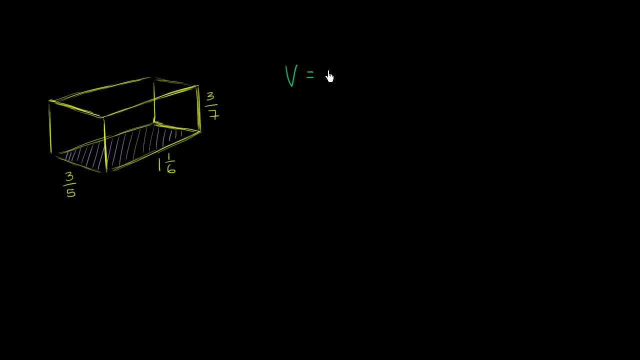 right over here. So sometimes you'll see volume is equal to the area of the base. times the height. Times the volume, Times the height. This right over here is the height And let me make it clear This is the area of the base. 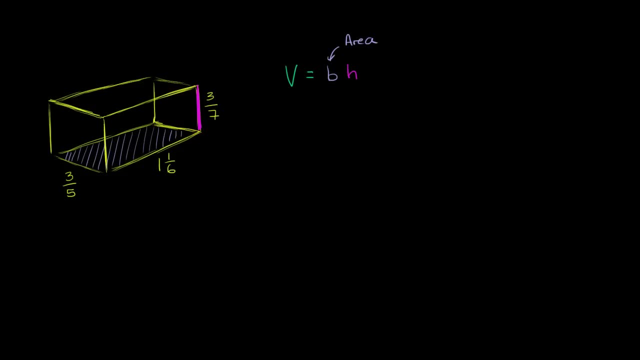 Area of the base times the height. Well, what's the area of the base? Well, the area of the base is the same thing as the length times the width. So you might see it written like that. You might see it written as area of base. 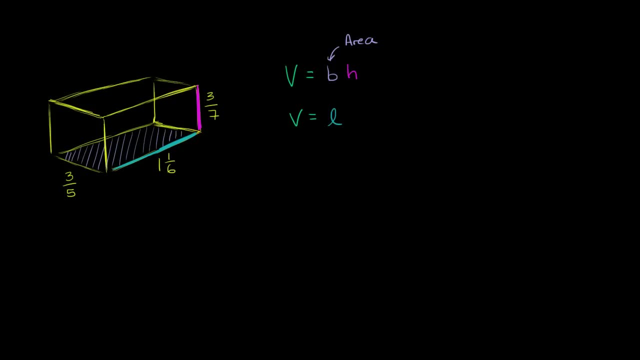 is going to be your length times your width. Length times width is the same thing as your area of the base. So that's that right over there, And of course you still have to multiply times the height, Or another way of thinking about it. 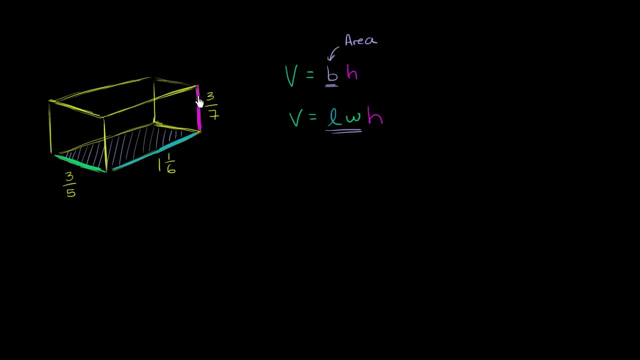 you're going to multiply your length times your width times your height. You're going to multiply the three dimensions of this thing to figure out how many unit cubes could fit into it, to figure out the volume. So let's calculate it. The volume here is going to be what's our length. 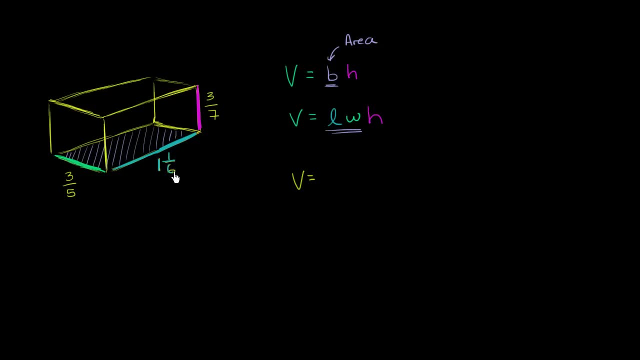 Our length is 1.. 1 and 1 sixth units. Now, when I multiply fractions, as I'm about to do, I don't like to multiply mixed numbers. I like to write them as improper fractions. So let me convert 1 and 1 sixth to an improper fraction. 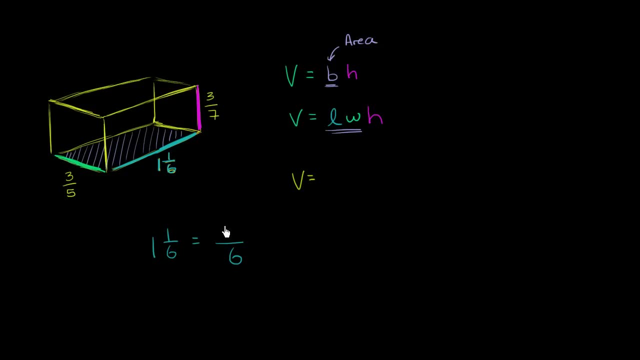 So 1 is the same thing as 6 sixths, plus 1 is 7 sixths, So this is going to be 7 over 6.. That's my length, Times 3 fifths. That's my width. So times 3 fifths. 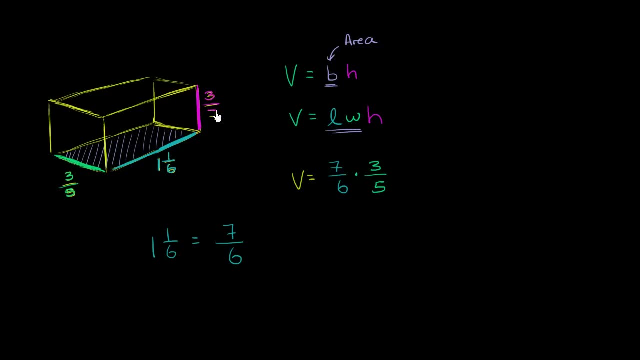 Times the height. Times the height, which is 3, sevenths. And we know when we multiply fractions, we can multiply the numerators. So it's going to be 7 times 3 times 3 times 3.. And the denominator: we can just multiply the denominators.